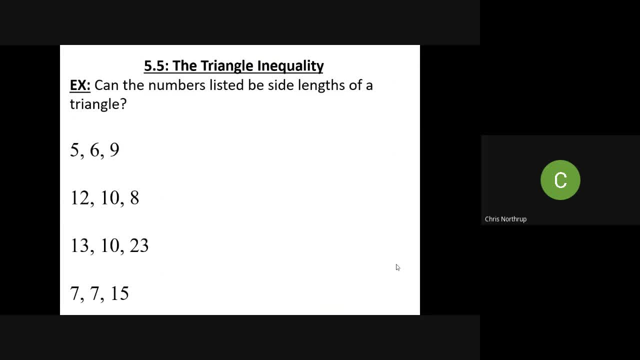 And someone asks you: can you form a triangle with these numbers being the side lengths? To do a quick check, you just look at the smaller numbers so that first triple 5, 6, 9.. 9 is the longest one, so let's check 5 plus 6,. 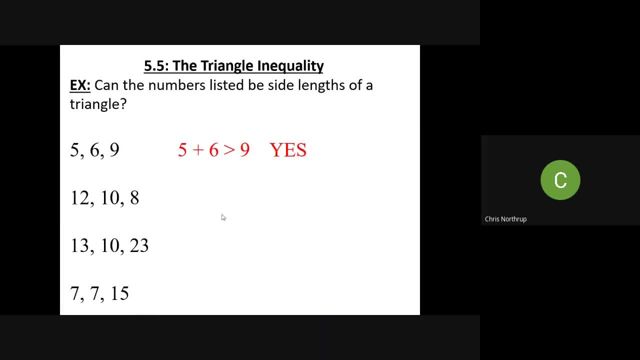 the smaller lengths add to more than the largest one. So, yes, you could form a triangle with those numbers being the side lengths. For the second triple there, 12 is the longest one and the two smaller ones add to more than that. 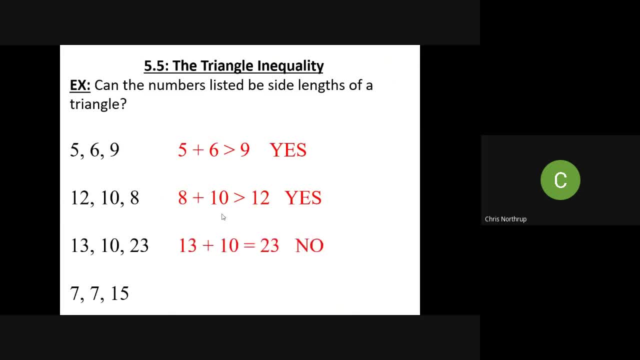 So yes, you could. On the third one, here you do not get more than- and it has to be more than- It can't be equal to, And we'll talk about this in class. but no, you couldn't make a triangle with those numbers. 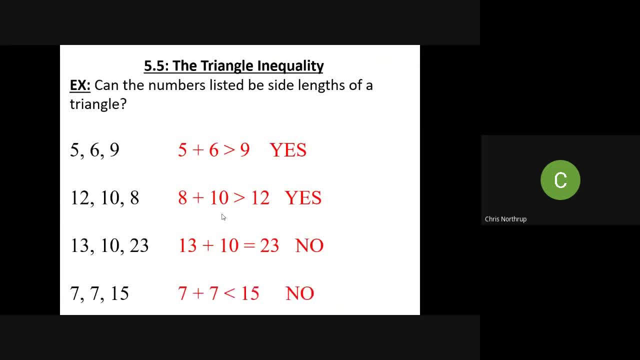 And lastly the two smaller ones, 7 and 7, they do not add to more than 15.. So no, you couldn't form a triangle with those numbers. The next part of this video: we're going to take a look. 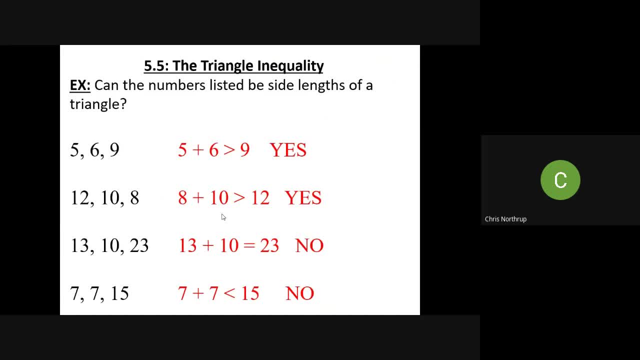 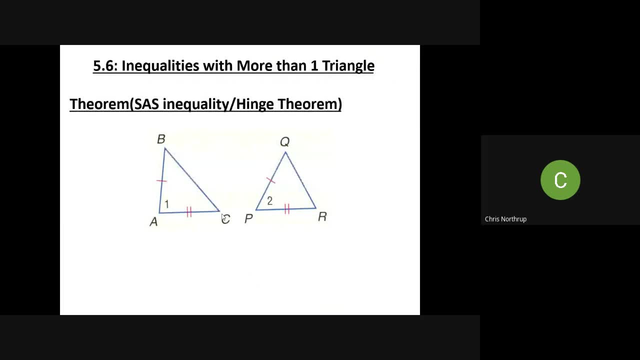 We're going to compare two different triangles, So this is a little different than what we've seen before. The first thing is called the side angle, side inequality. Some people call this the hinge theorem. So suppose you have these two triangles where you know that two pairs of sides are congruent. 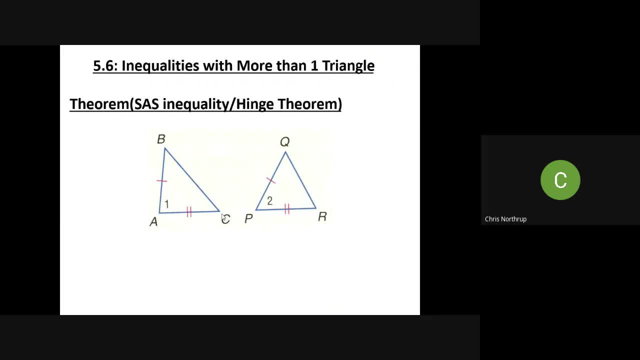 and you know what the measures of the angles are. Now, if we know that 1 and 2 are congruent, we know that the triangles are congruent by side angle, side congruence. But the question is, what if angles 1 and 2? 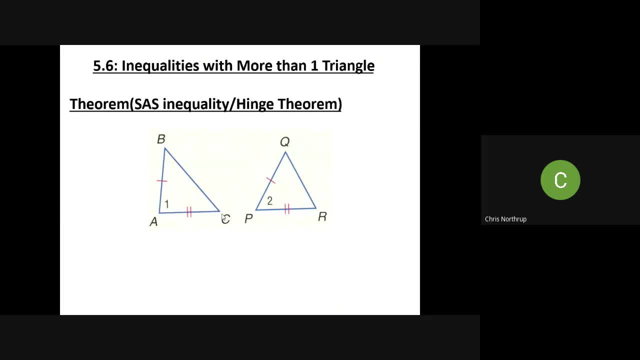 are not congruent, However, those angles compare. what will tell us how those sides compare? So, for example, if angle 1 was 65 and angle 2 is 48, since 65 is larger than 48, that would tell us. 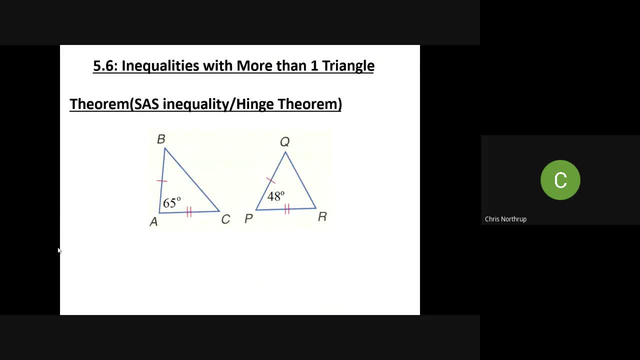 that BC has to be longer than QR. And if angle 2 was bigger, we would say QR is bigger than BC. But since we know that 65 is more than 48, we can make that conclusion that BC is longer than QR. 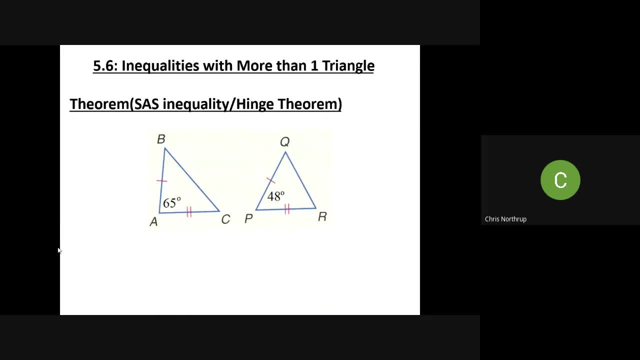 So keep in mind you have to know that AB is compared to PQ and that AC is compared to PR. If you have that and if you know how the angles compare, that will tell you how the sides compare. The converse of that is also true.